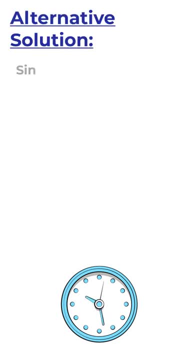 lot of problems. there is an alternative way to solve it. Since one hour movement of the minute hand is represented by 360 degrees, we can look at 12 numbers on the clock and each number on the clock is a number of minutes. To solve this challenge, we need to emphasize the fact that defective clock 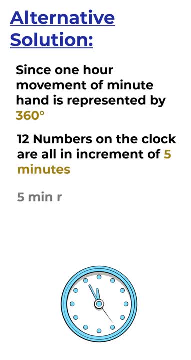 is an increment of 5 minutes. 5 minutes is represented by 30-degree angle, which is calculated as 360 degrees divided by 12, number which equals 30 degrees. So 65 minutes would be represented by 360 degrees for the full circle, plus 30 degrees for extra 5 minutes, which would 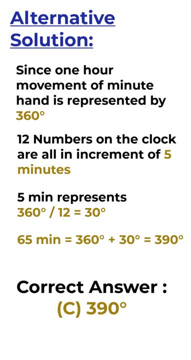 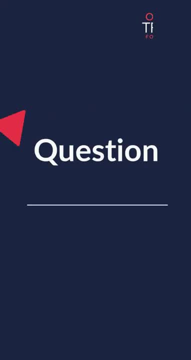 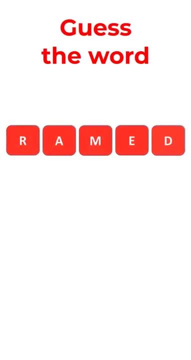 be 390-degree angle. Did you find other alternative solutions? Please make sure to share them in comments. Let's look at the question which you see on the test. very often You need to guess the word and you're presented with 5 different letters. On the screen. you see letters R, A, M, E, D. 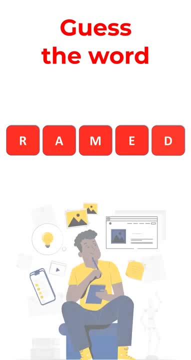 and you need to form a valid English word using these 5 letters. If you're trying to practice for the test, you might consider pausing this video and giving yourself a little bit of time to solve this challenge. If you're trying to practice for the test, you might consider pausing this video. 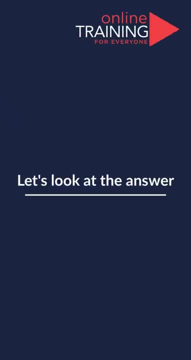 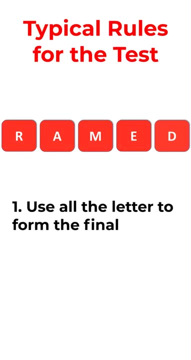 and giving yourself a little bit of time to solve this challenge. Every test is different, but typical rules require you to use all 5 letters and the final word that you form should match the number of letters that you see on the screen. A lot of times you might 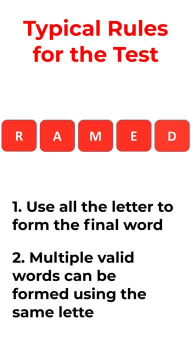 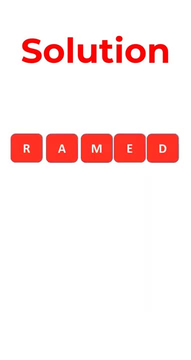 be able to form multiple words using the same letters. Ready or not, I'm going to move forward and reveal the final solution. The solution to this challenge is the word DREAM, which is spelled as D, R, E, A and M. Do you see any other solutions to this challenge? Make sure to post. 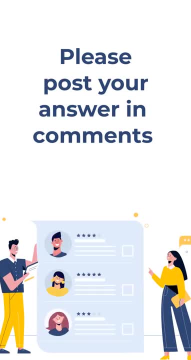 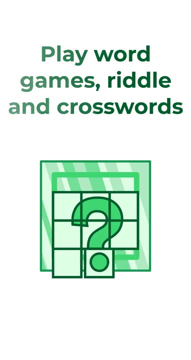 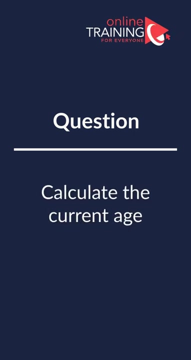 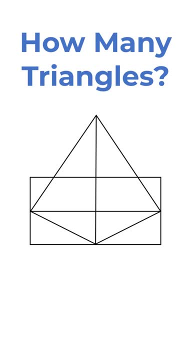 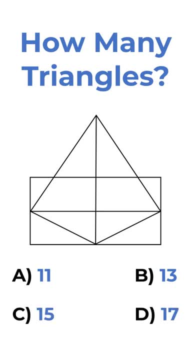 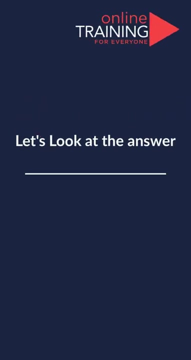 Choice C: 15. And choice D: 17. Do you see the answer? Consider giving yourself a little bit of time, maybe 10 to 20 seconds, to see if you can count all the triangles. Ready or not. I'm going to move forward and show you how many triangles did I discover? Tricky question. 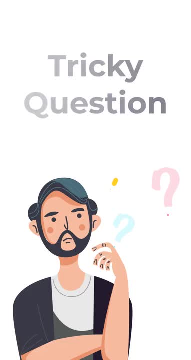 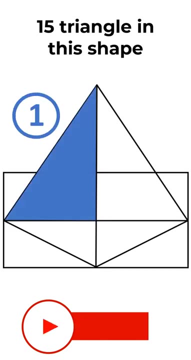 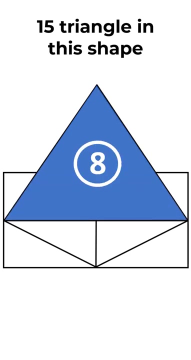 don't you think so? But I was very surprised when I counted 15 triangles in this shape. Let me go over and show all of them to you. Here's the first one, second, third, fourth, fifth, sixth, seventh, eighth, ninth, ten. 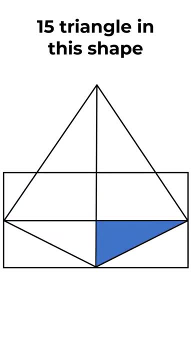 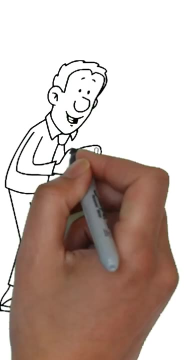 eleventh, twelfth, thirteenth, fourteenth and fifteenth. Do you see any additional ones? Please make sure to post them in the comment section of this video And, if you're getting ready for the assessment test, please make sure to check out the description for the link to the. 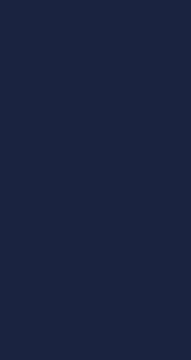 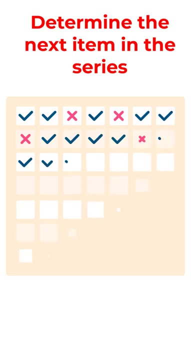 ebook that will help you to get ready. Very frequently on the test you might get a question to determine the next item in the series. We're looking at exactly this type of question here. You're presented with the series of three by three matrices. 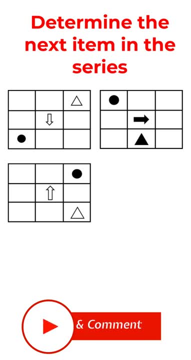 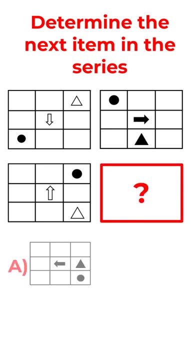 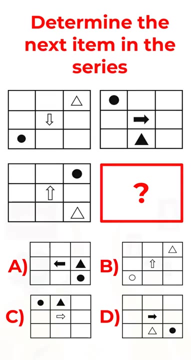 Each matrix has circle, arrow and triangle inside And your goal is to determine matrix number four in the series. You're presented with four different choices: Choice A, B, C and D. Take a close look and see if you can determine the pattern. Ready or not. I'm going to move forward. 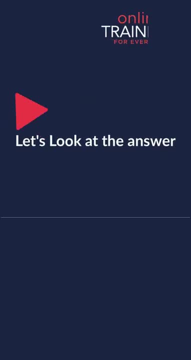 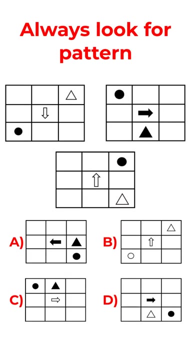 and share with you the correct answer, at least from my standpoint. When solving this type of challenges, my advice to you always look for patterns, And there are multiple different patterns here for each shape- Circle, for example, changes places, but always remains black, and 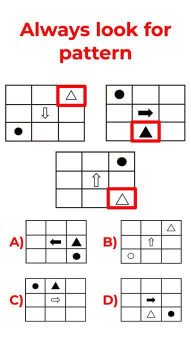 always filled with color. Triangle changes places in the matrix, but changes from filled with black color to non-filled with black border And arrow rotates counterclockwise. changes places in the matrix, but changes from filled with black color to non-filled with black border.